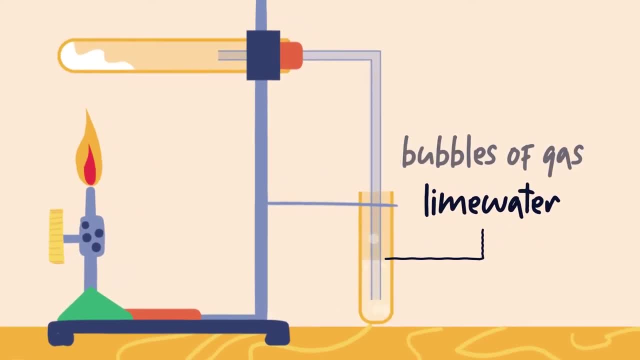 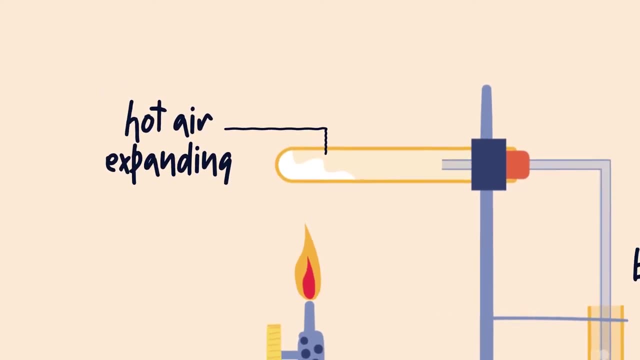 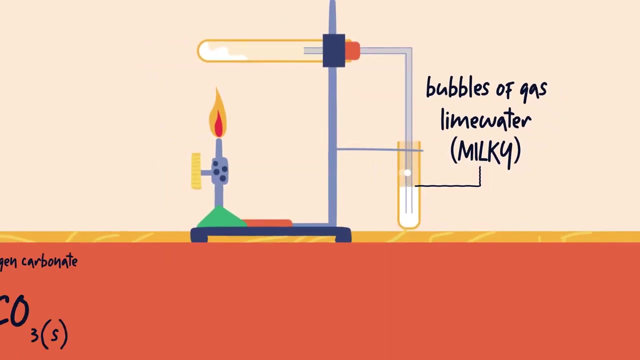 experiment On gentle heating, bubbles of gas can be seen in the lime water. This is initially due to hot air expanding in the test tube, but soon a steady stream of bubbles is seen that turn the clear lime water milky. This shows the carbon dioxide has been made as the hot 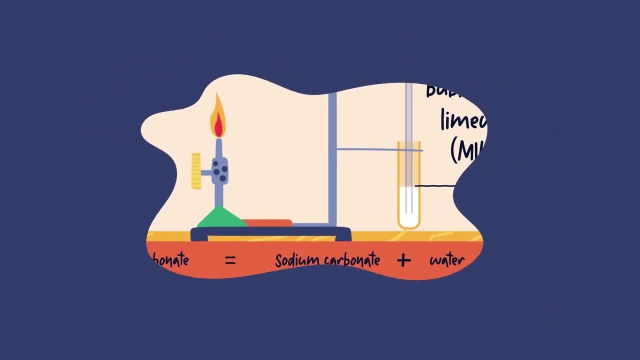 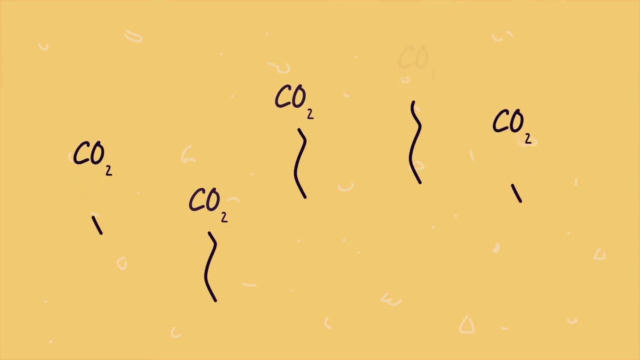 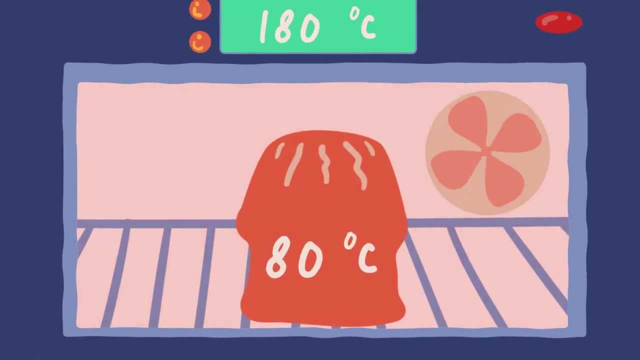 sodium hydrogen carbonate decomposes, So when it's a part of a cake sponge mix, the baking powder breaks down to release carbon dioxide gas, which expands and creates millions of bubbles to raise the cake mixture. This reaction begins at above 80 degrees centigrade and, as cakes are baked, at about 180 degrees. 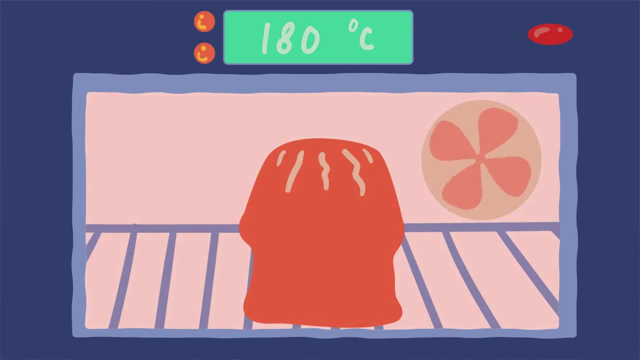 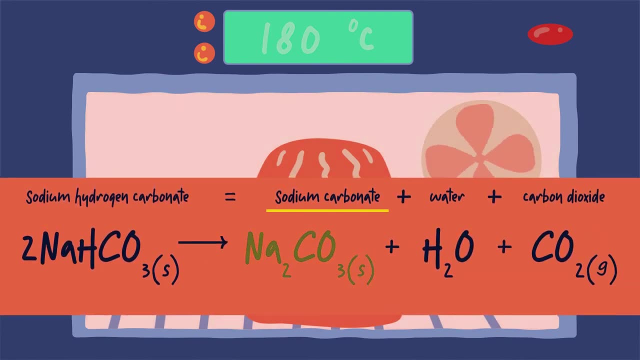 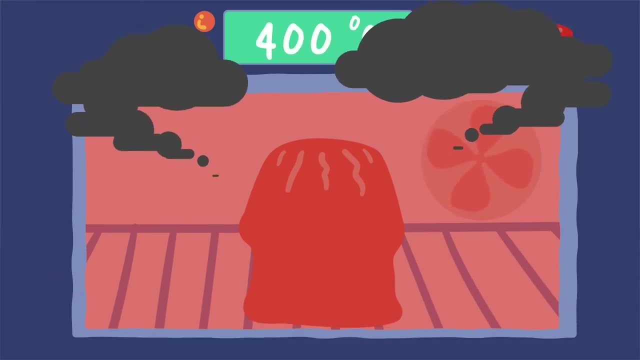 centigrade. this reaction proceeds easily. If you notice, the breakdown of sodium hydrogen carbonate makes sodium carbonate Na2CO3.. Sodium carbonate is quite stable to heat and only decomposes if heated above 400 degrees. centigrade Sodium carbonate is well above cake baking temperature, and so this reaction doesn't happen. 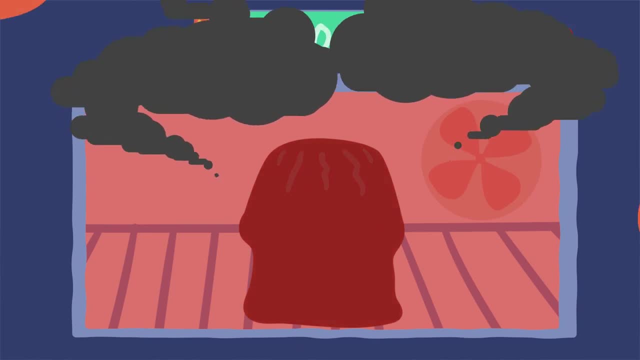 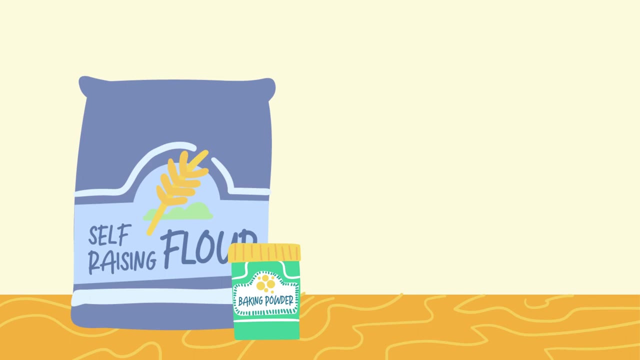 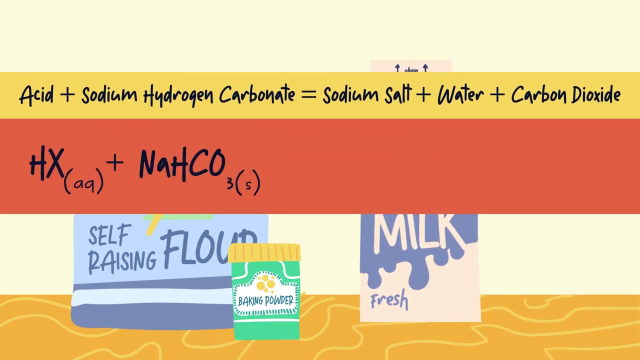 Otherwise the whole cake would thermally decompose. There is another way the baking powder- part of self-raising flour- can be used. This uses the chemical reaction that takes place between metal carbonates and acids: Acid plus sodium. hydrogen carbonate equals sodium salt plus water plus carbon. 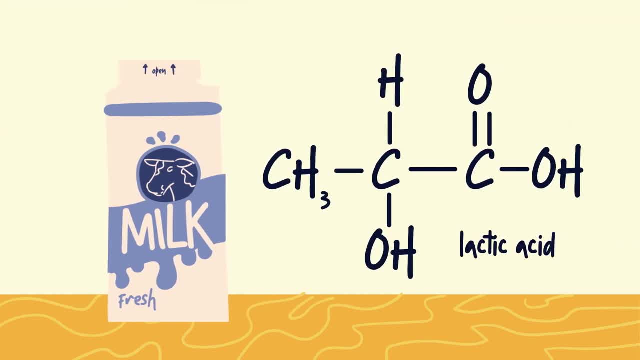 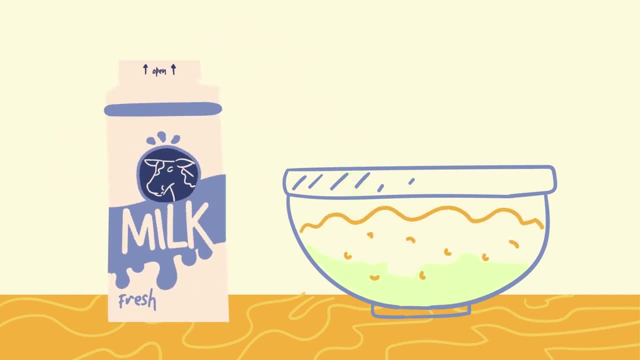 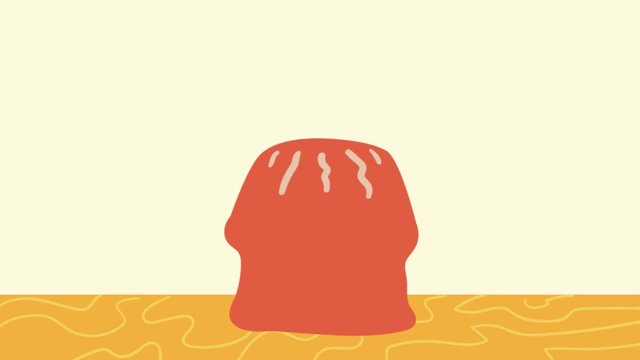 dioxide. When milk turns sour, lactic acid is made. When milk turns sour, lactic acid is made. If sour milk is used to make a cake mix, this begins the reaction to generate carbon dioxide before it's even placed in the oven. This can give a lighter baked cake as more carbon. 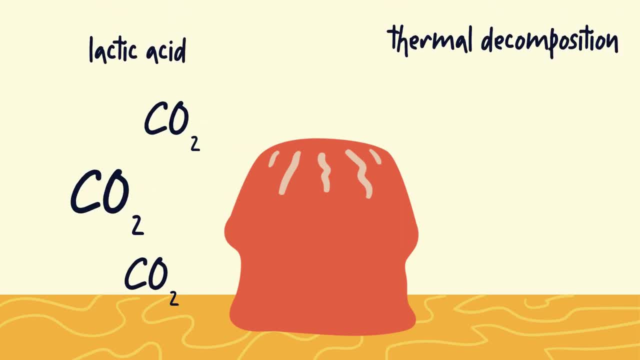 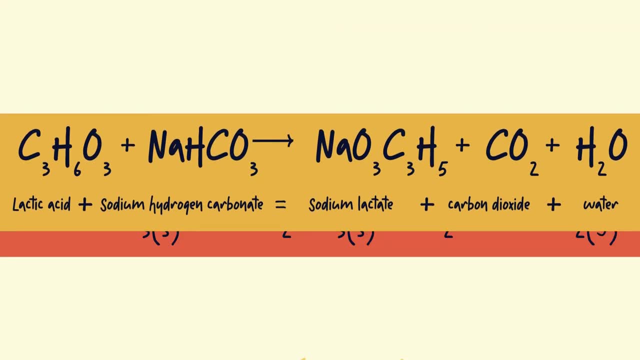 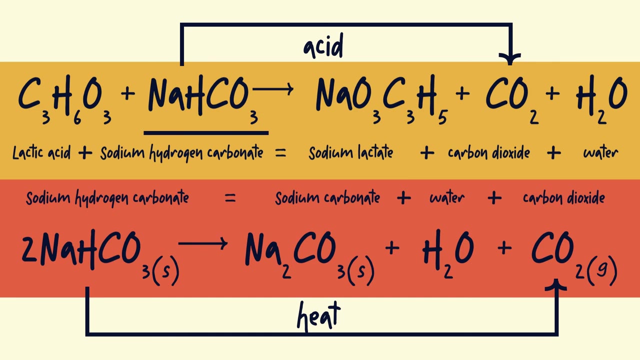 dioxide was made than just relying on thermal decomposition of sodium hydrogen carbonate, and is also a way of using up sour milk. If the two reactions are compared, you can see that the one importance is 아니야, and other things run wild. Sodium hydrogen carbonate can generate more carbon dioxide when treated with acid than when heated. 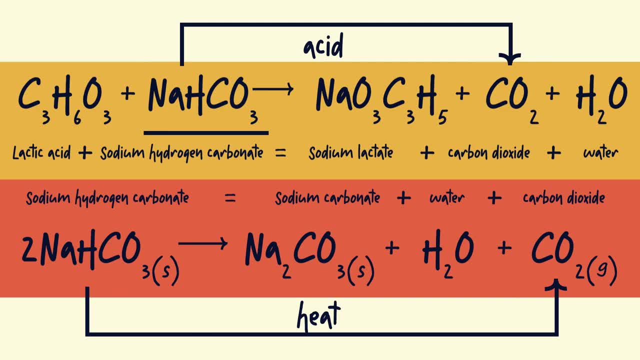 Sodium hydrogen carbonate can generate more carbon dioxide when treated with acid than when heated. If you don't have glutinous değiş這些 playing a role in your breads, you can also use wings and meric or wafers to cheese. the eggs and chocolate점 quiereurs.